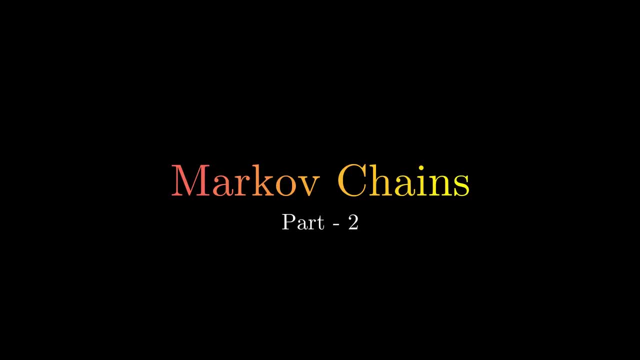 previous video first and then continue with this one. The link will be available in the description and will appear in the cards right now, So I hope you have the basic knowledge First. I'm gonna take a very simple Markov Chain For the sake of simplicity. 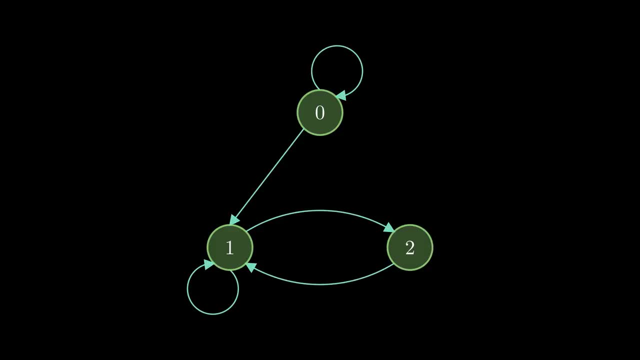 I haven't written the transition probabilities on the transition arrows. Just remember: if there is an arrow from state A to state B, then it means that there is a transition error between state A and state B. So there is an arrow from state A to state B, Then it means that there is a transition error. 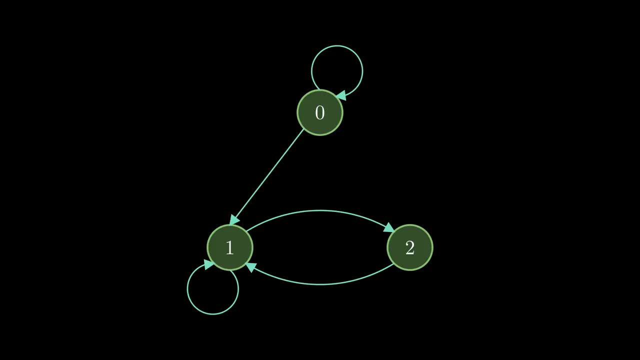 between state A and state B. This means that there is a transition error between state B and state B. Then it means that there is an error between state A and state B. there's a non-zero transition probability from state A to state B. 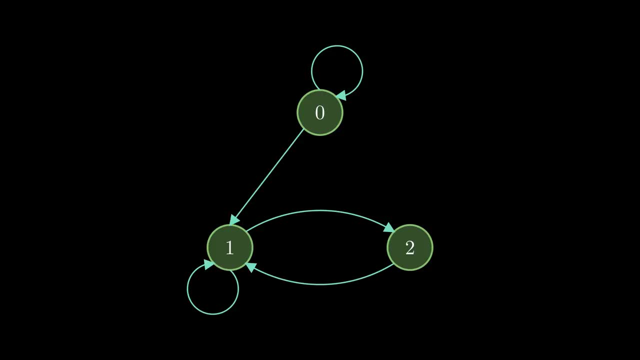 And obviously the sum of the outgoing probabilities from any given state is one. Now focus on the state zero. We are gonna perform a random walk starting from state zero and we will try to find if something interesting is going on For the first couple of times. 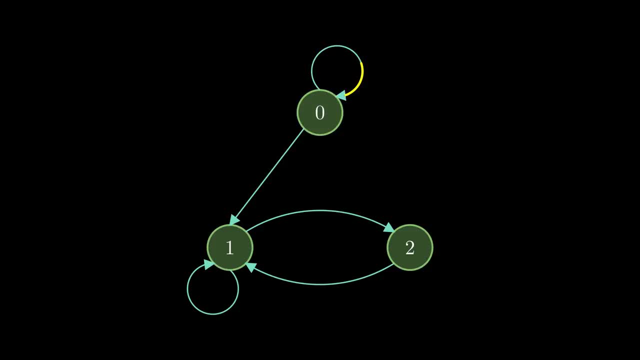 we are looping in state zero itself, But as soon as we leave state zero and go to state one, then state two and et cetera. now there's absolutely no way to go back to state zero. It might happen that in some random walks. 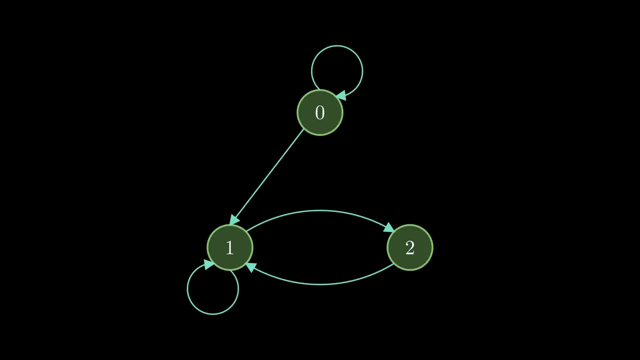 we never leave state zero, but it might also happen that we leave state zero and we never come back again. So the probability of revisiting state zero in a random walk that started from state zero to state zero is less than one. We don't know for certain whether we are gonna come back. 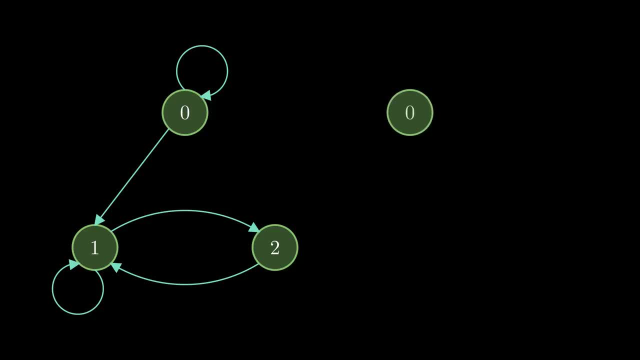 This type of state, for which the probability of coming back to itself is less than one, is called a transient state. Now let's focus on state one. Here's a random walk starting from this state. We can clearly see that after some time, 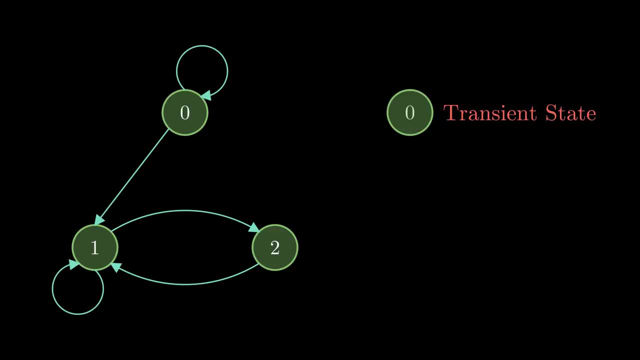 we are bound to revisit state one, So in this case, the probability of coming back to state one is one. This type of state is called a recurrence state. The same is true for state two also. Look at this random walk starting from state zero, and convince yourself. 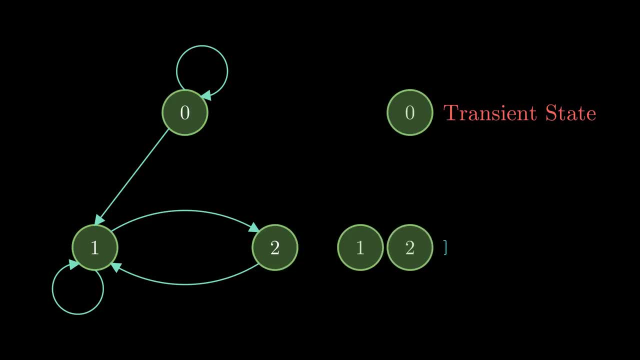 So both one and two are recursive recurrent states. okay, now let's try to understand why state 0 is not recurrent. well, this is because there's no way to go from state 1 or state 2 to state 0. in this type of situation, where some states are unreachable from others, we say the. 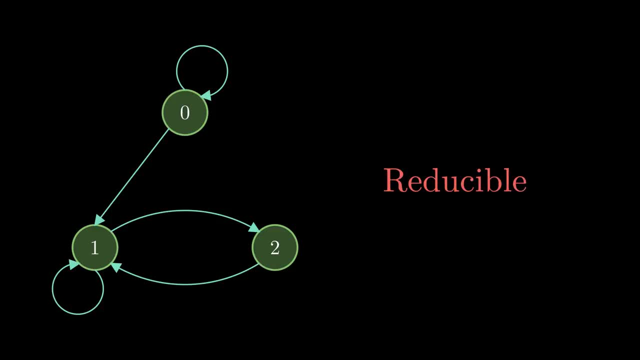 Markov chain is reducible. now I'm gonna add a single edge connecting state 2 and state 0. this time we can easily see that every state is reachable from every other. consequently, state 0 has become recurrent. this type of chain where we can. 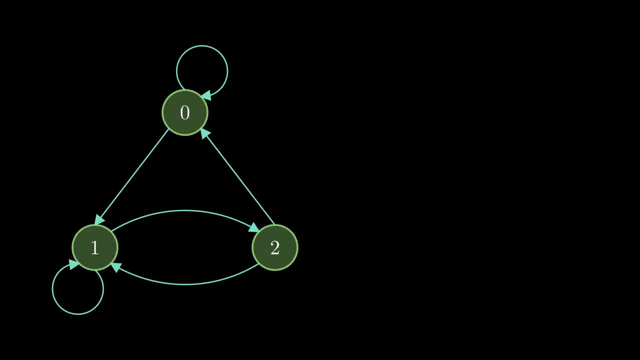 go from any state to any other is called an irreducible chain. now let's go back to our original Markov chain. you might wonder why they named it reducible. well, it's probably because it's not a reducible chain. it's called a. 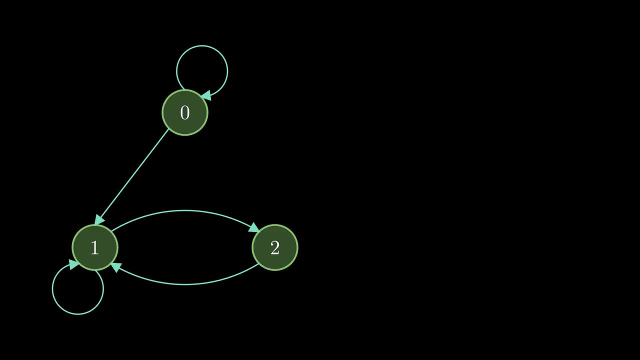 2019 chain. it's probably because we can divide or reduce this chain into smaller chains which are irreducible. let's delete the transition from state zero to state 1. we can imagine two Markov chains here. the upper one contains only one state and it's recurrent, and hence it. 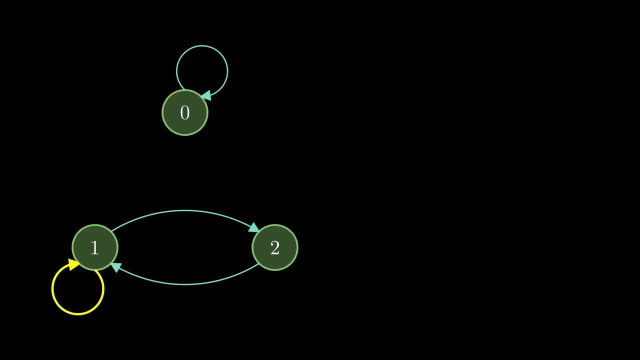 reducible. the bottom one contains two states, and every state is reachable from every other state, hence it's also irreducible. okay, now I'm a changed my identity class today, so why is a state 0 unreducible? okay, now I'm a changed my identity class today, so why is a state 1 irreducible? 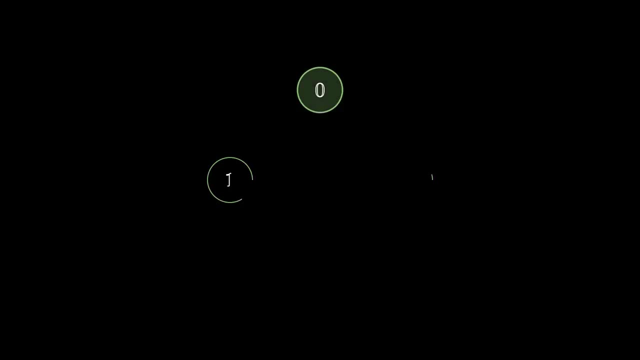 okay. so why is a state 0 unreducible? Now I'm gonna take a slightly bigger Markov chain. Some of you might be familiar with this. It's famously known as the Gambler's Ruin, But let's not get overwhelmed by the name. 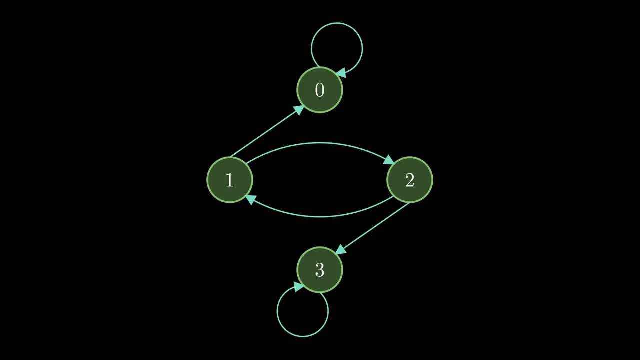 Just consider this as a regular Markov chain. What we want to find here is which states can communicate with each other, And by communication I mean both way communication. Let's focus on state zero. If we start from state zero, we can't go to any other state.